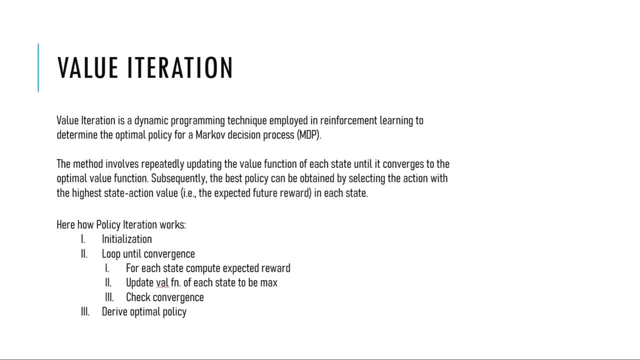 For each action using the current value function. Next we update the you know value function for each state to be maximum expected future reward of you know all the action. And then we keep checking the convergence by comparing the you know change in value function for each state to a converge you know convergence threshold. After that we basically derive our policy. So so what we do inside this part, we loop over each state and select the action that maximizes the expected future reward. 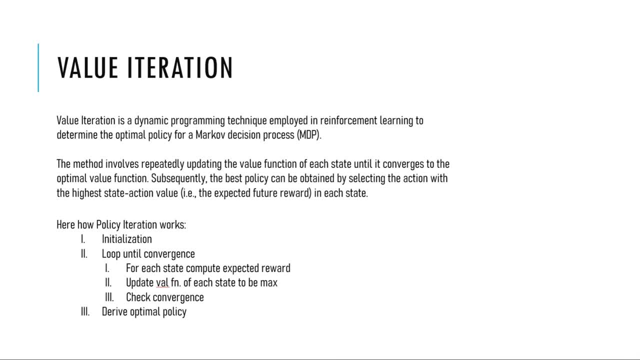 Okay, and that is the action with the highest state action value. So what we do, we first initialize, we run the loop, we update our you know value function- and it should be you know max- and we keep checking the older value and the latest value of our you know value function So that I mean whenever the convergence you know hit, I mean the given threshold, we will get to know and then we will derive that whatever the maximum we have found there, it will be maximum. 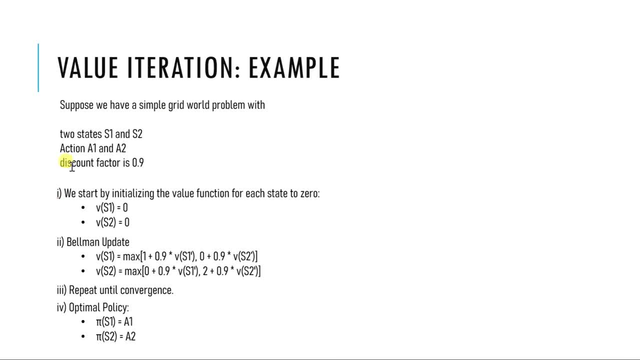 Our optimal policy. Okay, now let's understand it through, I mean, example. Okay, so basically, suppose we have a simple grid, grid wall problem with two states, S1 and S2.. Okay, and we have two action, A1 and A2, for each state. Now, for each state you will be deriving, you know, the reward for each state action pair, Like we, you know, derived in policy iteration algorithm. Same way, let's say: this is our. 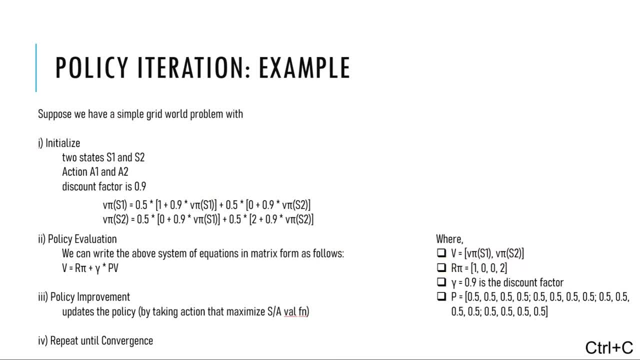 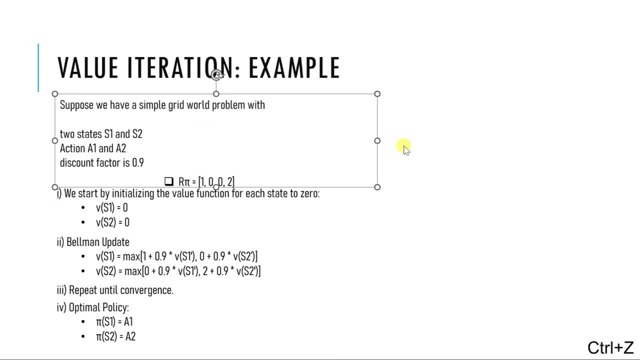 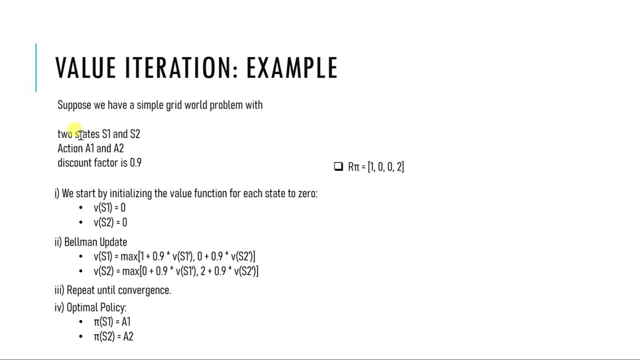 Okay, so I'm just copying it into our value iteration algorithm. So let's say: this is our, this is our reward function. Okay so so since we have two state, two action, so there will be four tuples right. So for every combination we have our reward. So for state one, action one, it will pick one. for state one, action two, it will pick zero. for state two, action one, it will pick zero. 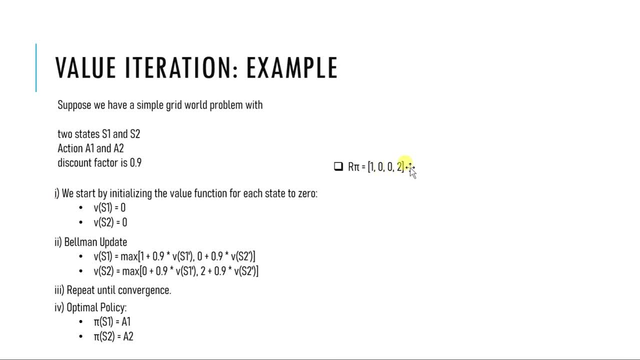 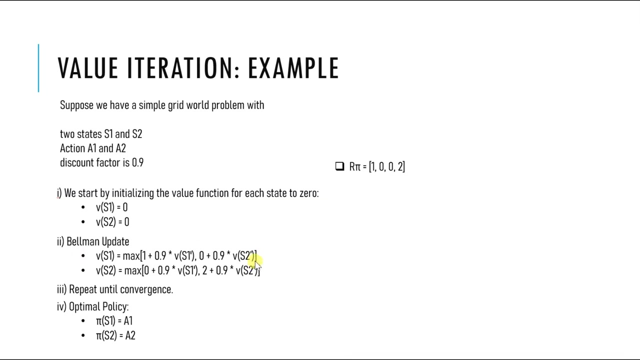 For state two, action two, it will pick two: Okay, and our discounting factor is 0.9.. So first, what we do? we initialize. I mean we start by initializing the value function for each state to zero- Okay, like this: V of S1 to zero, V of S2 to zero, Okay. and then what we do? we apply the Bellman optimality equation for value function- Okay. so the first equation that you see here represents the value function for state one: Okay, and 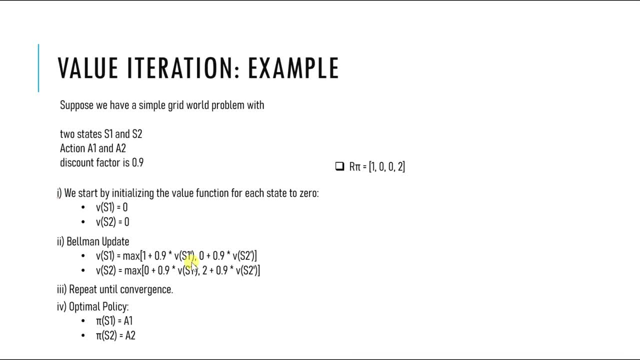 here the value of S1 is the maximum of sum of, you know, immediate reward one, as well as and the discounted value of the next state, S1 dash, And the sum of immediate reward zero and the discounted value of next state, S2.. So both are given Okay, and in the second equation obviously it is similar, So it represents the value function for state two. Here the value of S2 is maximum of the sum of immediate reward, zero, Okay, and the discounted value of next state, S1 dash. Similarly, 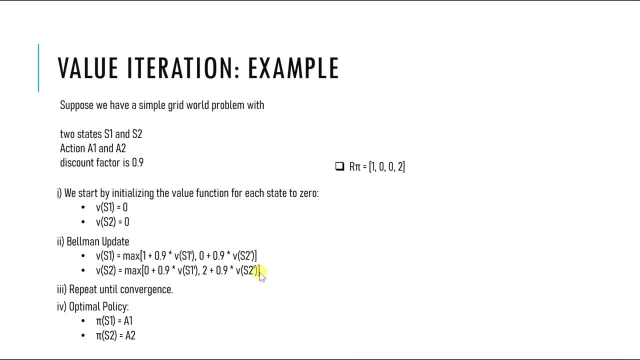 the sum of immediate reward, 2, okay, and the discounted value of next date as 2 dash. So these equations are used to, you know, I mean obviously for the purpose of value iteration, to find the optimal value function and the optimal policy for given MDP, okay. 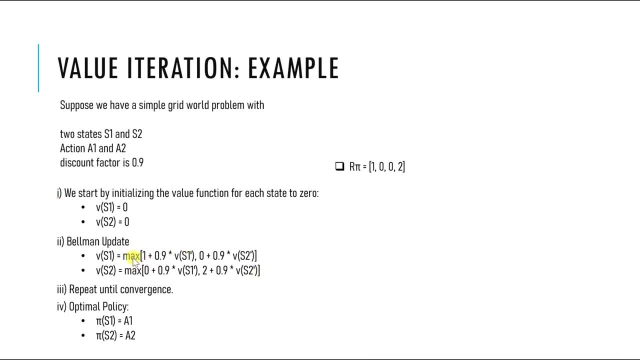 So basically there is also only different. we see here with the- you know policy iteration algorithm. okay is the. you will see that there is a extra, I mean thing that is happening, that is max, okay. So basically, what max denotes is: max denotes the maximum operator over all the possible. 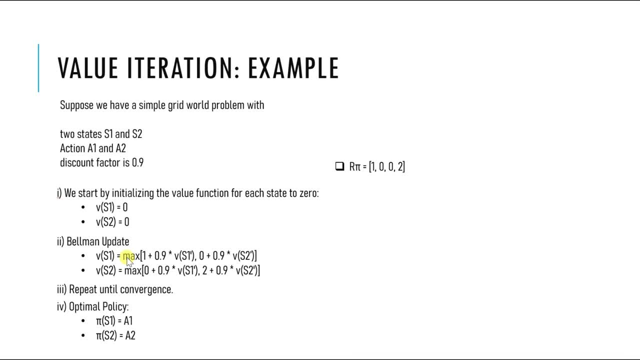 action in the current state and S1 and S2 dash okay, denoting the neighbor state of S1, S2 respectively. So whatever the you know maximum will be from the neighbor state as well as the current state. it will pick that whichever is the maximum. 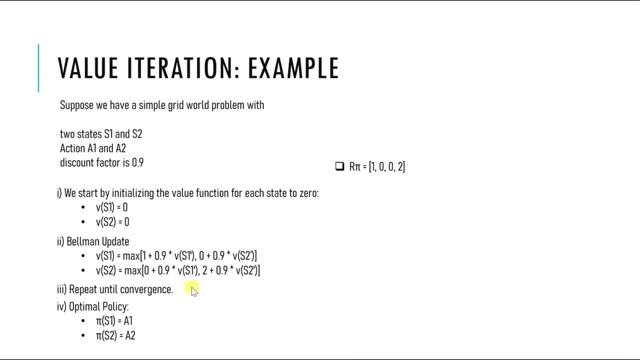 And then what we do? we do iteration. So basically in this step we repeat the. So in each iteration we update the value function for each state based on the updated value of its neighbor state. okay, And then we apply the optimal policy.